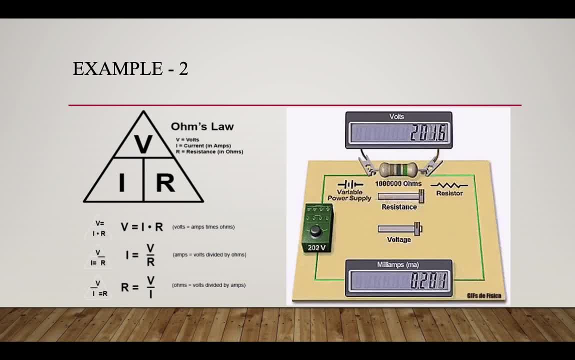 changing. so this physical system is a circuit. we will use this equation to calculate the current in the form of equations using ohm's law. v is equal to ir. so v is equal to ir is the mathematical model of this simple circuit. now we are going to cover more examples in 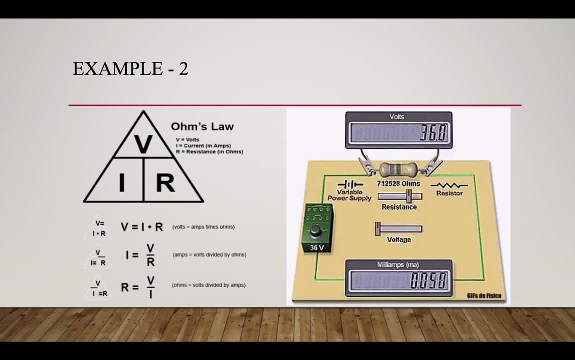 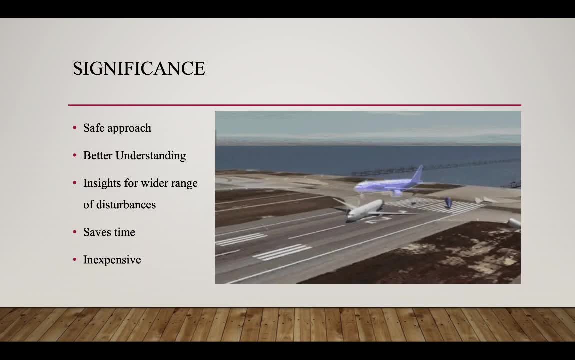 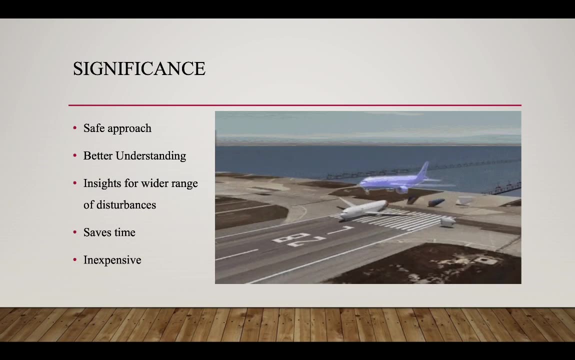 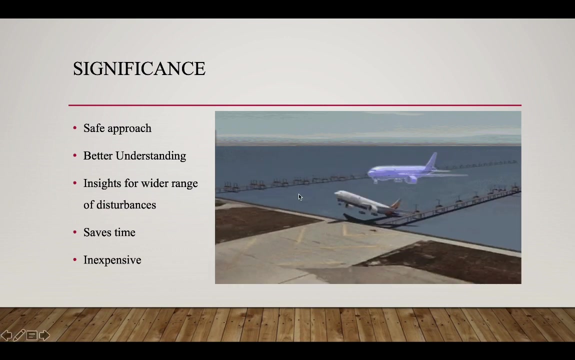 which you will get a better understanding in three cases. first of all, we will see what is the significance of this mathematical modeling. it is a very safe approach to go to calculate first the mathematical model, then go for the real situation. now take an example of an aeroplane you can see here in the video. this is an aeroplane, if you assume you have. 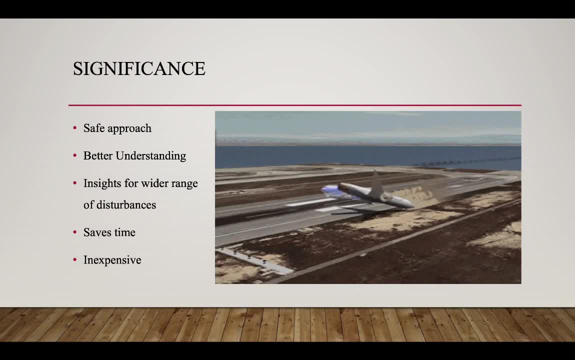 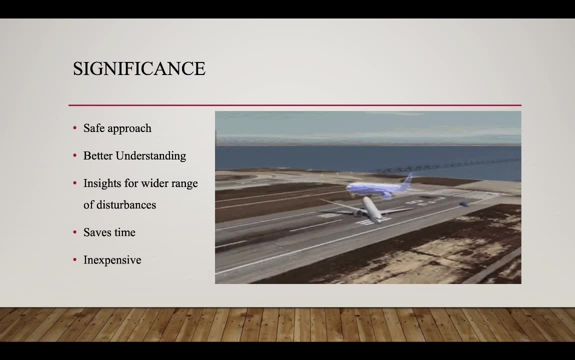 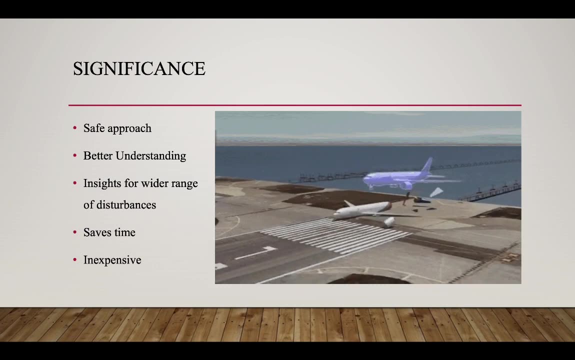 driven its mathematical model and you know what are the inputs and outputs in it, how much force it will be stable on applying, how much force it will be unstable. will it have a vibration level? Now for that you can calculate everything. after you have calculated this, you can learn. 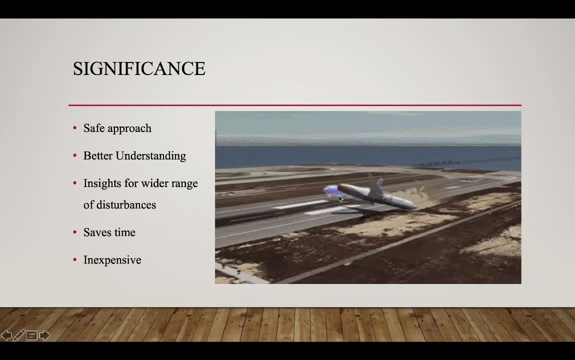 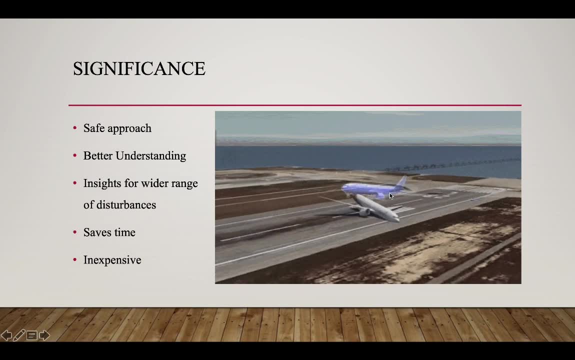 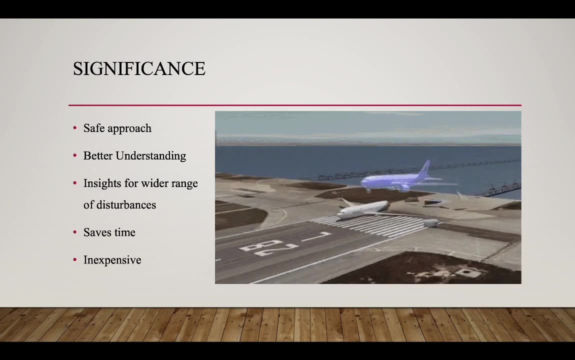 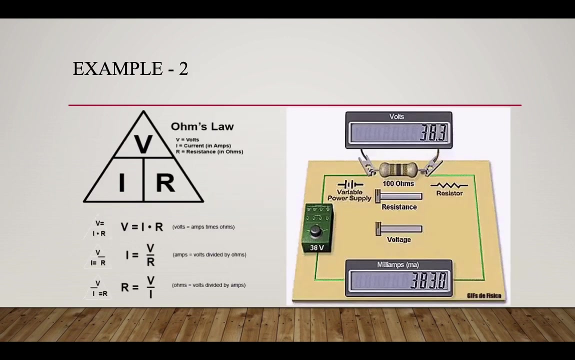 how this blue thing looks like. but if you work without mathematical modeling, directly, without any paper work, without any equation work, if you make a system directly, then it might crash and that system might fail. this is not just an example of this, but look at this example. you are aware of this if you find this example or if you have done it yourself. 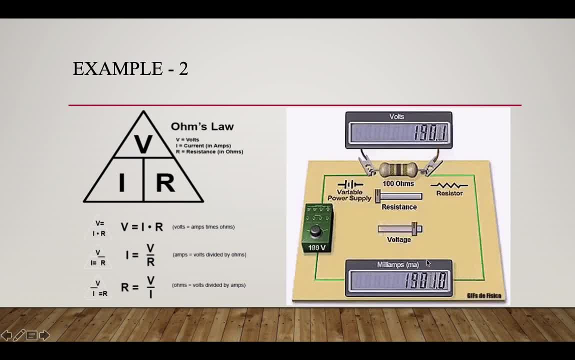 you know that this is a simple circuit, so you know which wire you have used, how much mm wire you have used, how much watt resistor you have used. you know all this, so from here you can find out what is the safe voltage level, what is the safe resistance level, 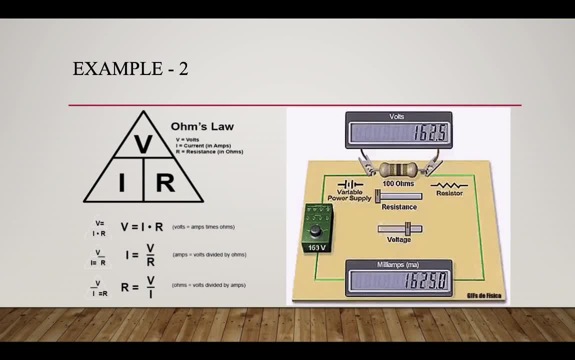 what will be the current flowing in the circuit. you can find out all this so you will know at what voltage current level is, how much will be and how will be the safety of my system. like you know the wire, suppose you have used 1 square mm wire. 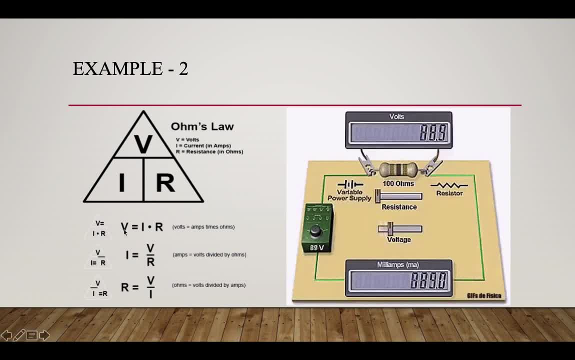 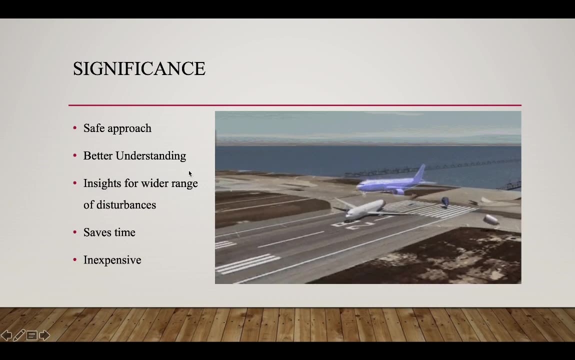 so you know how much current it can handle. from here you can find out how much voltage you can give in it so that your system remains safe, so that your circuit does not get damaged or burn. this gives you a better understanding. you can understand the system well. 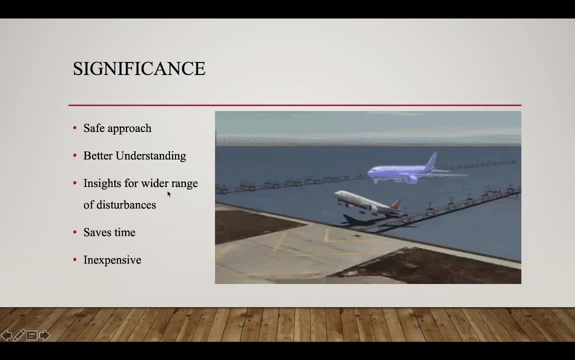 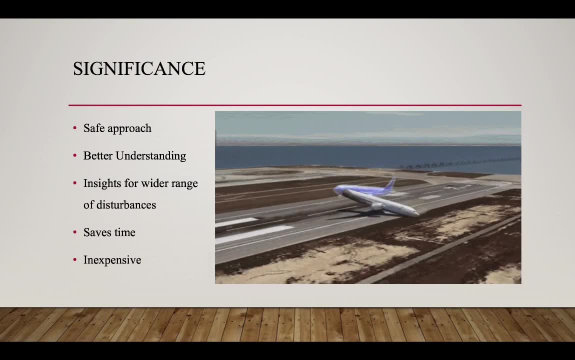 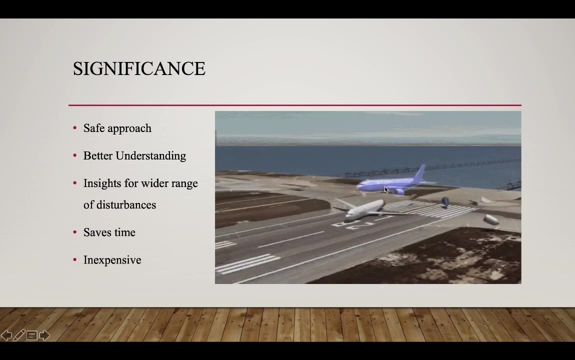 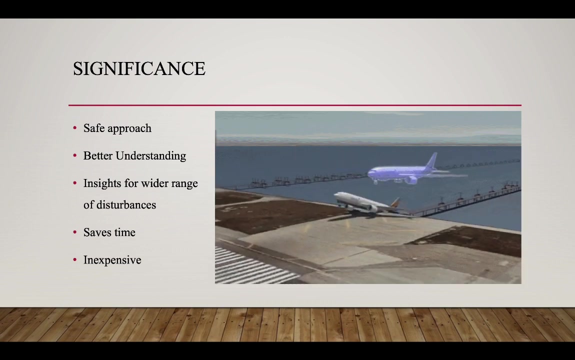 it gives you insights for wider range of disturbances. what does this mean? whatever is your real situation, there will be some disturbances, which we can call inputs or disturbances. suppose an aeroplane was flying and you got a vibration. what is that vibration? it is a disturbance. so how the system will behave on that disturbance. 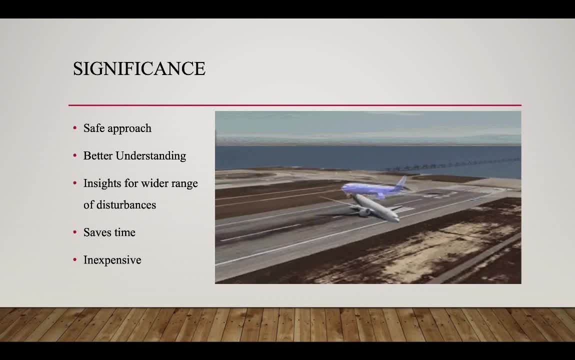 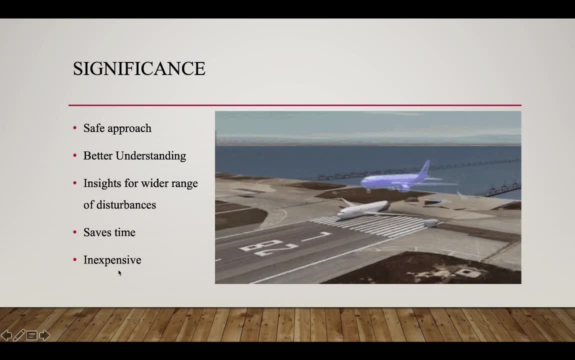 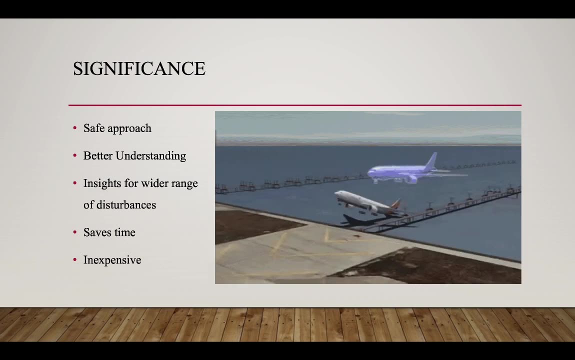 you can calculate all this if you have a mathematical model. it saves time, it is inexpensive. why is it inexpensive? because there is no cost in making a mathematical model. you can write it in the form of an equation. but if you want to create a real situation, if you want to make a real model, 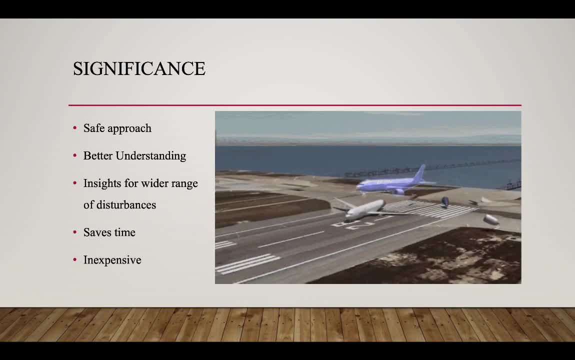 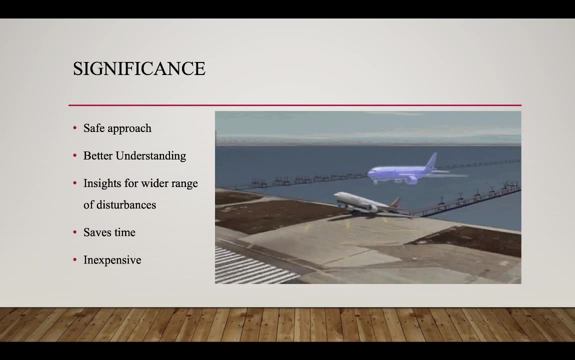 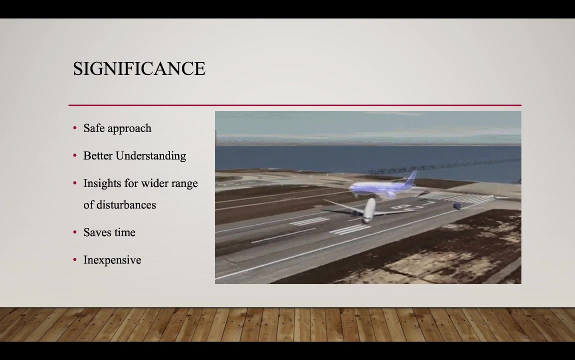 then it costs you a lot and after costing, if it fails or gets destroyed, then all your money will be wasted. so that is why mathematical model is a real model, but in form of equation. whatever you are going to make, it will be ready in the form of equations. 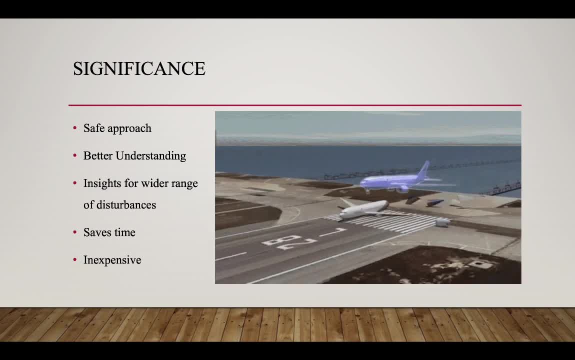 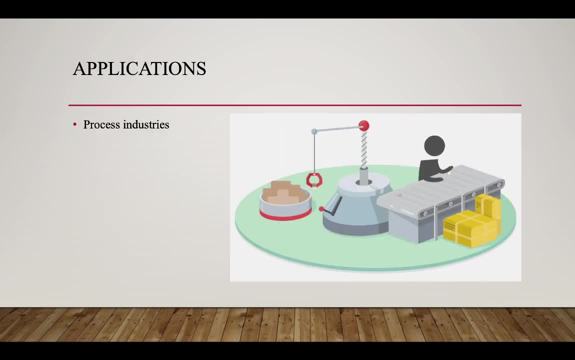 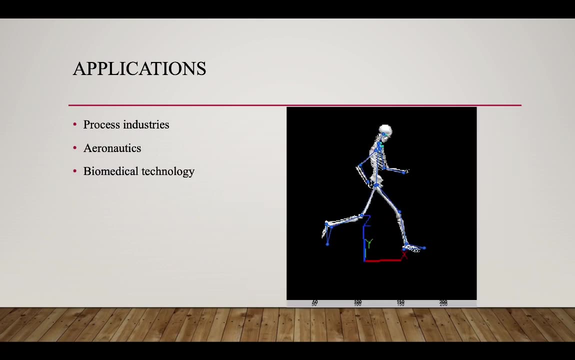 and we can analyze it in the form of equations and we can see the same behavior there. these are some of its applications. it is an application in the process industry. it is in aeronautics- we have already discussed in aeronautics. it is in biomedical technology. 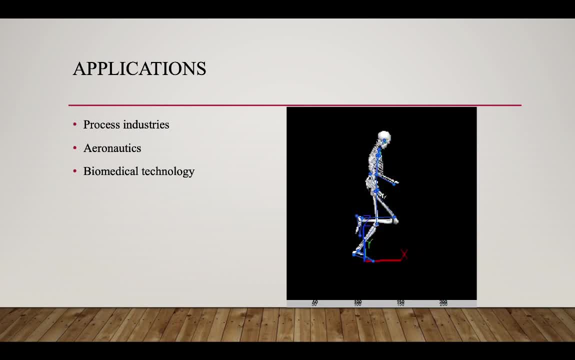 now see corona, corona is going on. you made a vaccine. you are not doing all this because it is not safe. what will be its behavior? we don't know. so first what we do, mathematical model is made, that mathematical model for different inputs, what kind of output it generates. 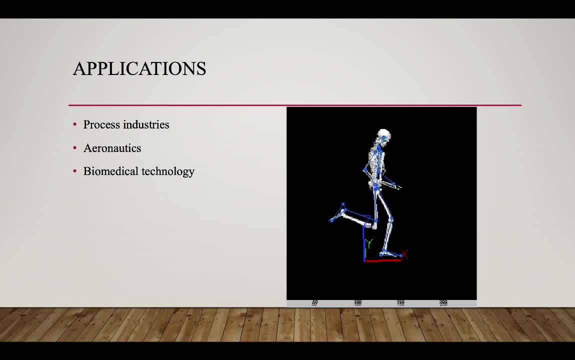 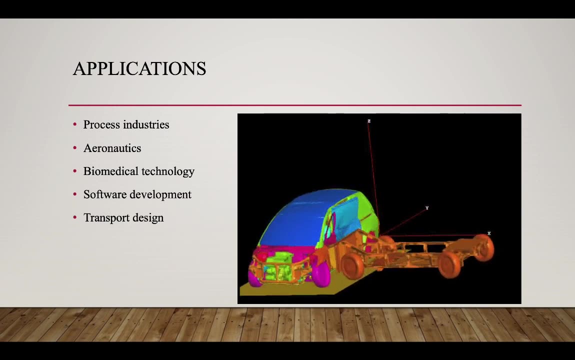 what kind of behavior we get after all that study. then its human trial starts. so in the same way, any equipment in biomedical technology, in today's time, for software development, for transport design, you should know how much impact you are driving. if the car collides somewhere, how much safety will remain. 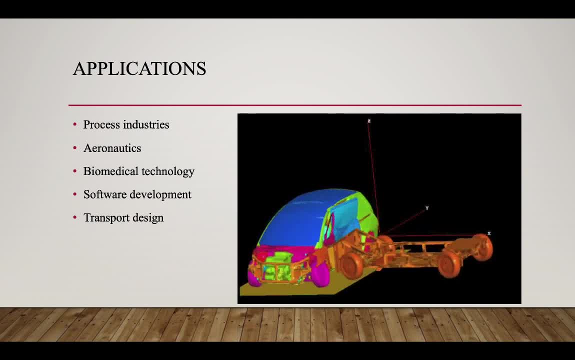 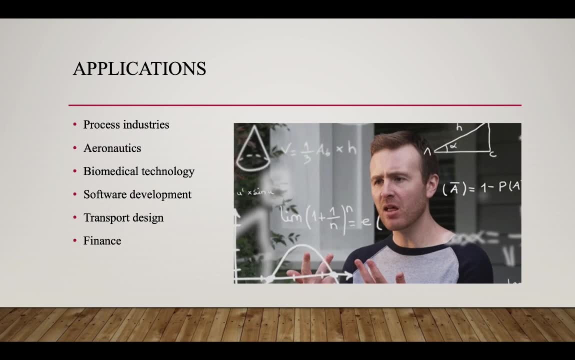 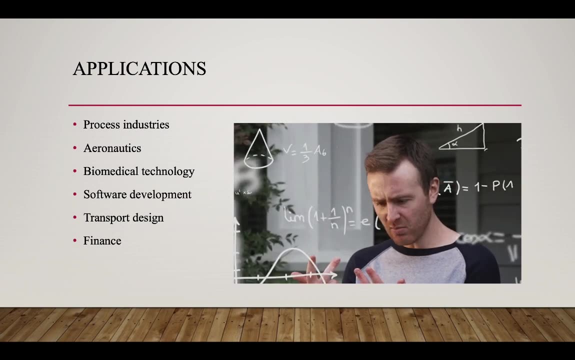 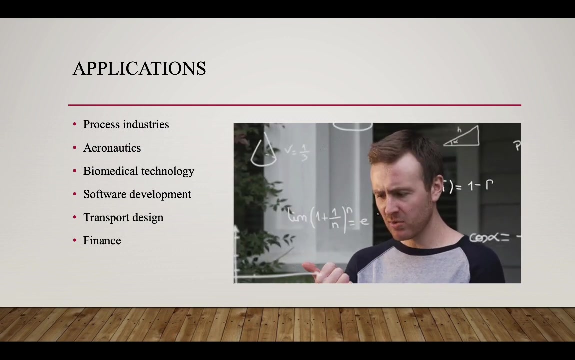 the man sitting inside. we can calculate all that through mathematical modeling. similarly, in finance, its application is now: you calculate interest, you calculate compound interest. you get all this in the form of a formula, the mathematical model of the real time situation. so it makes things very easy if you are asked to calculate interest. 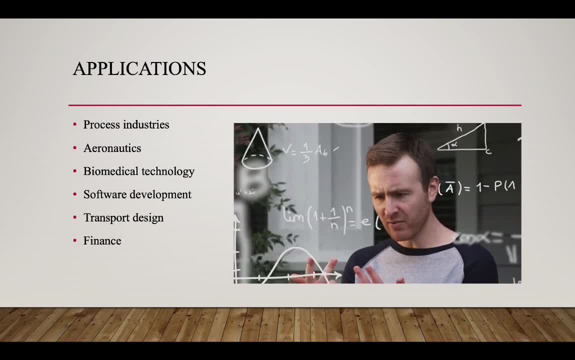 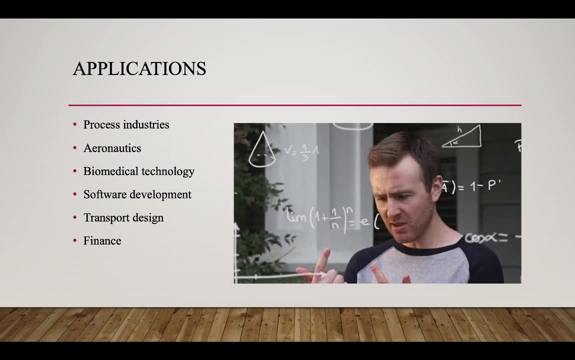 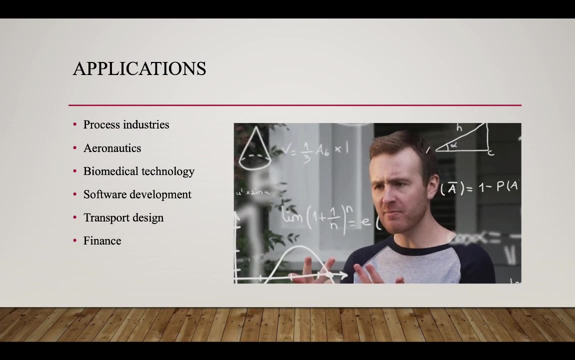 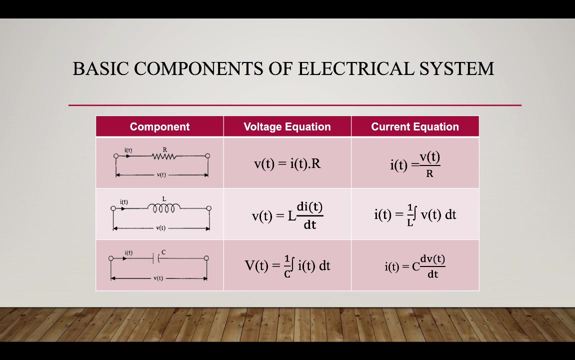 then you have the formula. so very fast you can calculate, and very easily. so all this is possible because of mathematical modeling. so almost every field has its application. so the main applications we have discussed here. now we will talk about electrical system. we have taken an example of electrical system. 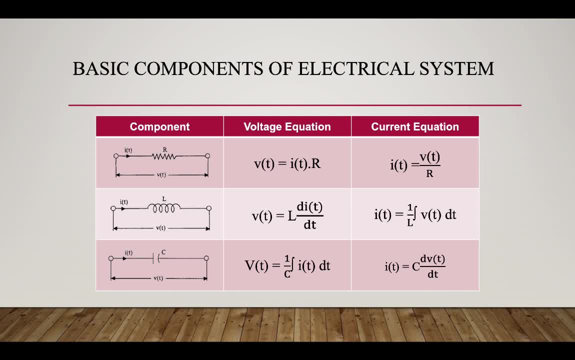 it has three basic components: R, L and C. any electrical system has three basic components. there will be three basic components: R, L and C: resistance, inductance, capacitance and what will be the voltage and current: voltage across these components and current through these components. 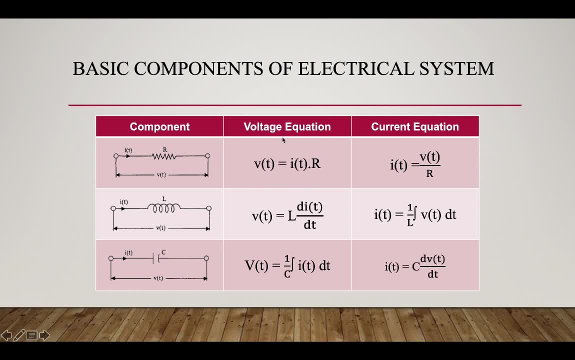 by ohms law. ohms law told us a resistance. what will be the voltage current through it? we can calculate through ohms law in the same way by Faraday law we can calculate the current across the capacitor and inductor through it. now a big circuit is made. 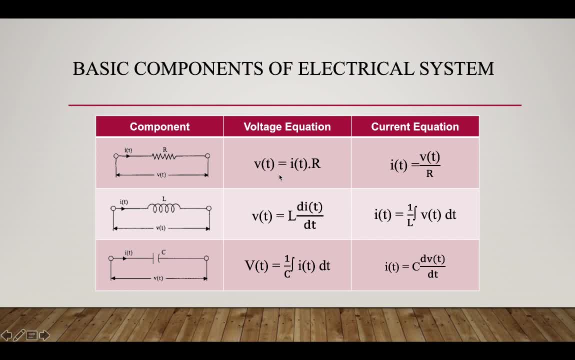 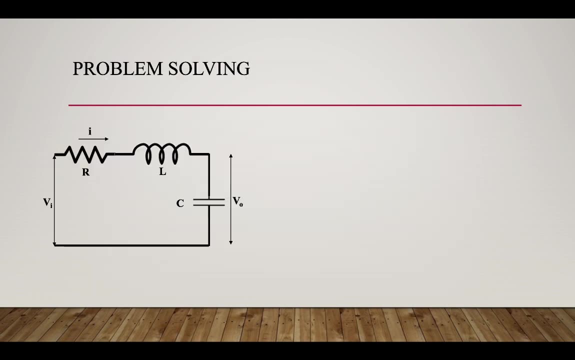 from all these components there we will put the values of these components and create a mathematical model. you will get questions in your exams. normally you are getting for mathematical modeling like. this is simple RLC circuit. there is a simple RLC circuit. there is input voltage, there is VI output voltage. 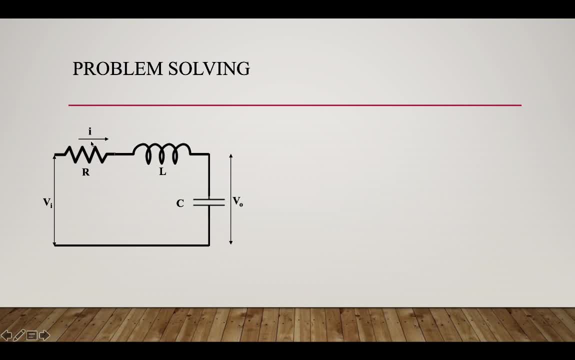 there is V0 across the capacitor, current is flowing through the circuit. there is value of R, resistance, there is value of L inductor. C is the value of capacitance. now, this circuit, this equation VI, is equal to RI plus LDI, DT plus V0. this is nothing but. 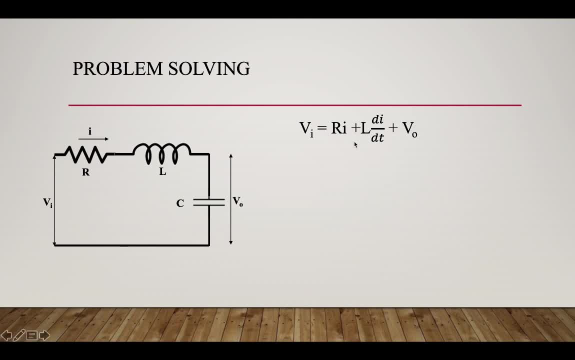 from the KVL Kirchoff's voltage law. algebraic sum of all the voltages in the circuit is equal to 0. this is the source. all these are my loads. source: voltage is equal to. voltage is across all the loads. so this we have across the resistor. 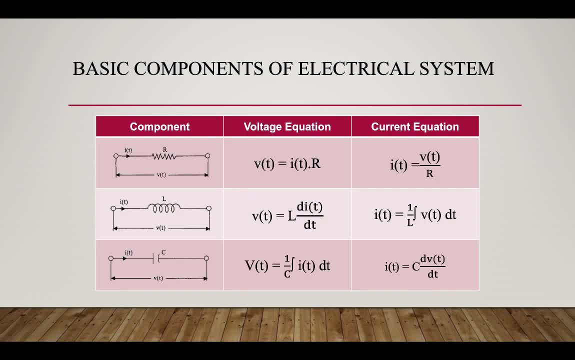 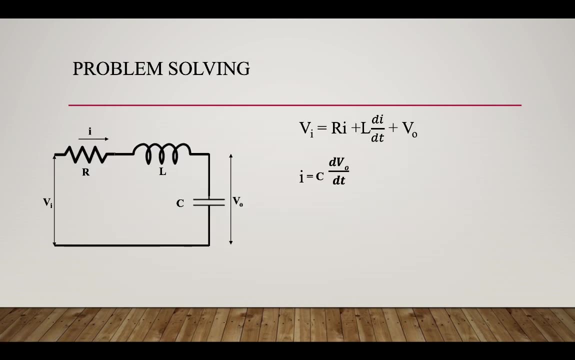 we have already seen that across the resistor voltage will be current will be across the inductor voltage will be capacitor voltage. we have applied, see the formula- current will be CDV0 by DT, and if we put the value of I here then we will get a relationship. 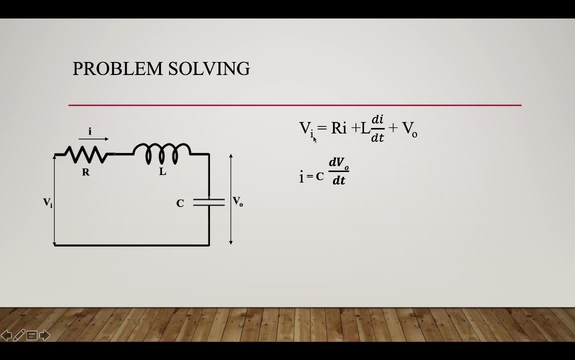 between the output voltage and input voltage. between the output voltage and the input voltage, we will get a relationship. see this, I have simplified it and here, in the form of differential equation, we have got an equation which is telling the relationship. This is the mathematical model of this circuit and we will use it to calculate the value of resistance capacitor and the output voltage of the circuit. 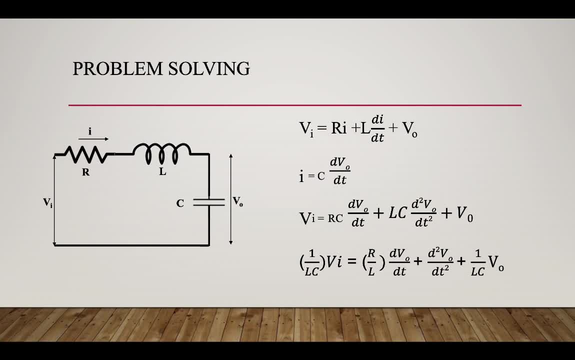 We will simplify this further. because differential equations are difficult to solve, We will take the Laplace equation and change it to algebraic equation. Algebraic equations are easy to solve. We have taken the Laplace equation. This is the relationship between the output voltage and the input voltage in Laplace form. 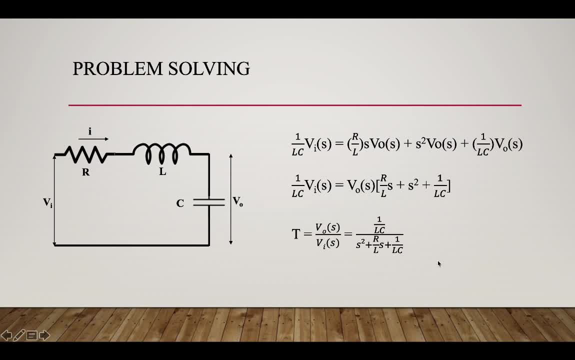 This is also called the transfer function. This is also known as the transfer function of the system. This was the example of the electrical system. Now we will take the example of the mechanical system. Before that, we will know the basic components of the electrical system. 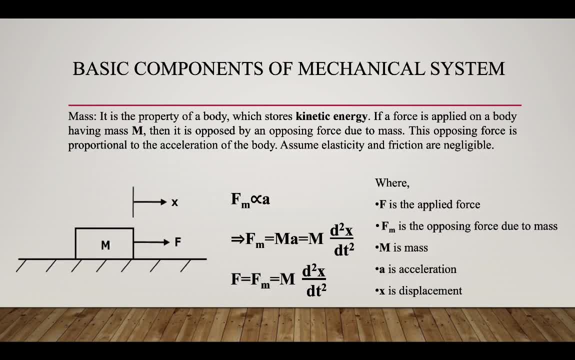 There are basically three main basic components: Mass, spring and dashboard. Mass spring and dashboard. So first of all, mass. Mass stores energy in the form of kinetic energy. If you apply force on any mass, there will be some displacement. 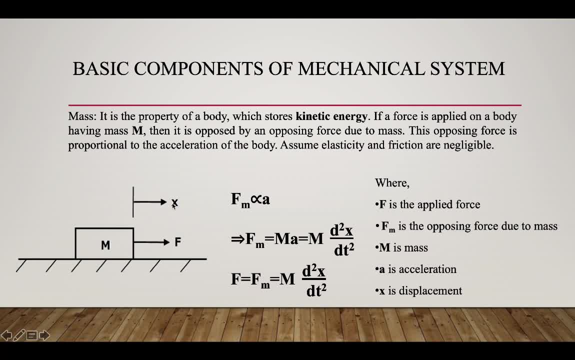 It will move, And how much it will move depends on the force. Acceleration is nothing but the double derivative of the displacement. So what have we done? Using Newton's second law, F is equal to MA, And in A, instead of acceleration, we have put D square, X by DT square. 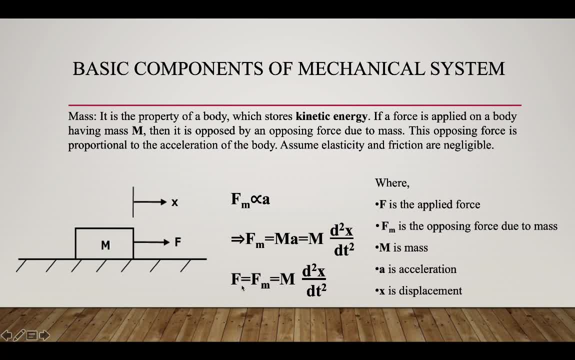 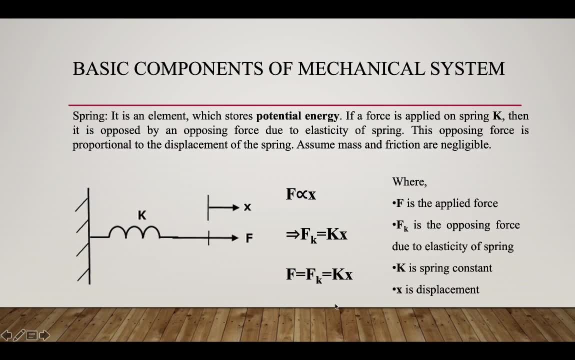 which is the double derivative of the displacement. So we have got a formula: F is equal to MD square X by DT square. Similarly for spring, we know from Hooke's law: F is proportional to X. It will move according to the force applied. 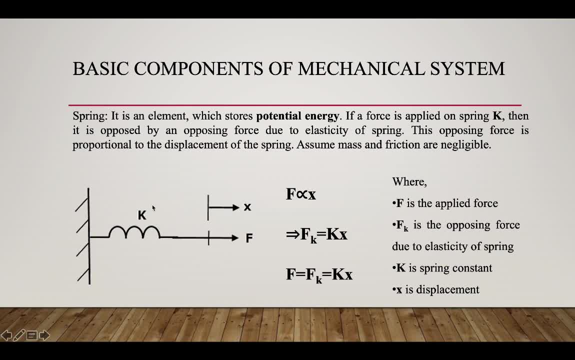 And who will stop it? Its spring constant K. It will oppose the movement. So from Hooke's law, F is equal to KX. We have got this relationship Between input force and output displacement. Similarly in the case of friction. 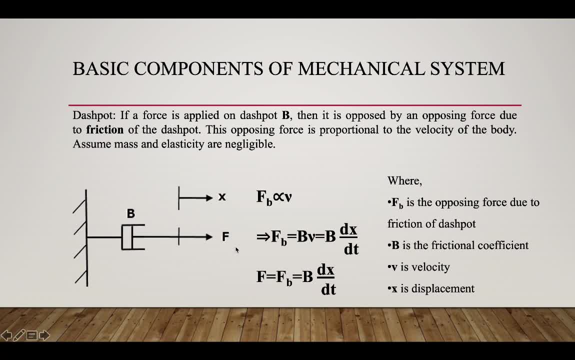 the force applied will be proportional to the velocity which is the derivative of, which is the first derivative of this displacement. So we have got the relationship. F is equal to B, DX by DT. These are the three main basic components for a linear system. 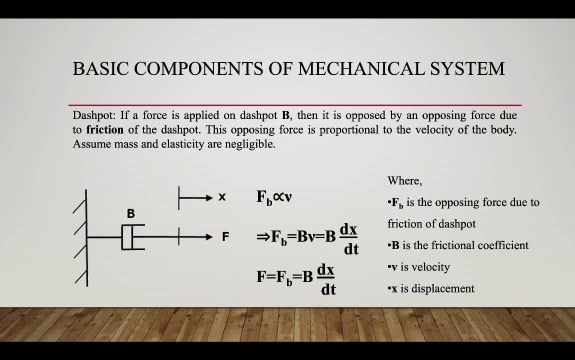 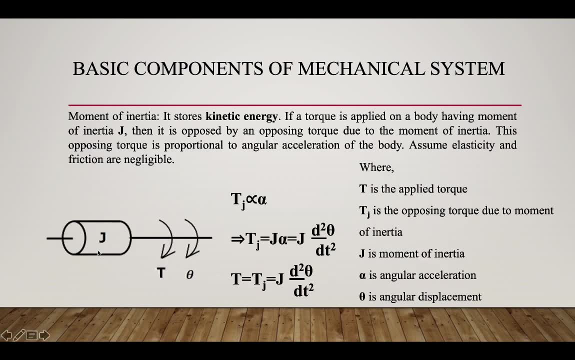 Similarly for a rotational system. we have similar three components, But instead of force there will be torque. See this. Some of the terminologies will change. The rest of the system will remain the same. The principle is same, But the motion there is linear. 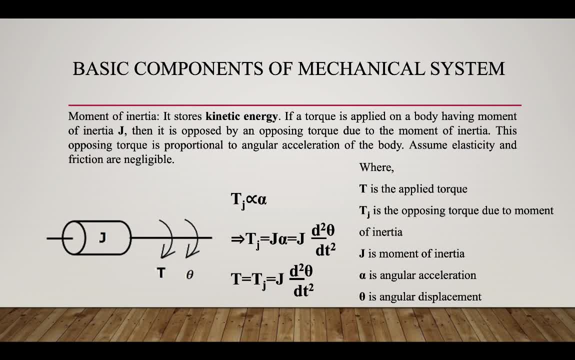 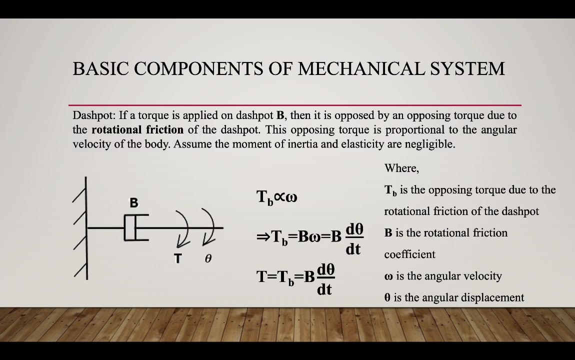 Here it is rotational. So there we were calling it force, Here we will call it torque, There we were calling it X. displacement, Here is the angular displacement, theta: Angular acceleration, Angular velocity. Similarly for spring, Similarly for dashboard. 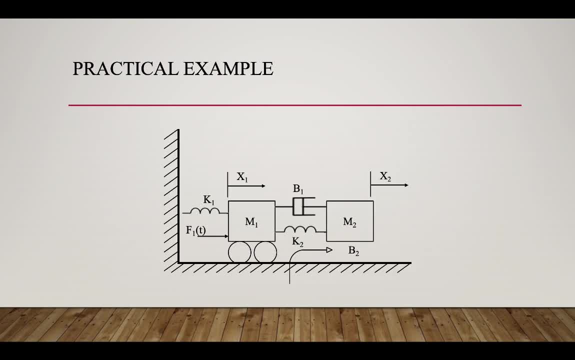 Here we will see an example of how to solve for the mechanical system. Here you can see that there is M1 and M2.. There are two masses, There are two springs, There is one dashboard. There is friction here. Now you are applying force from here. 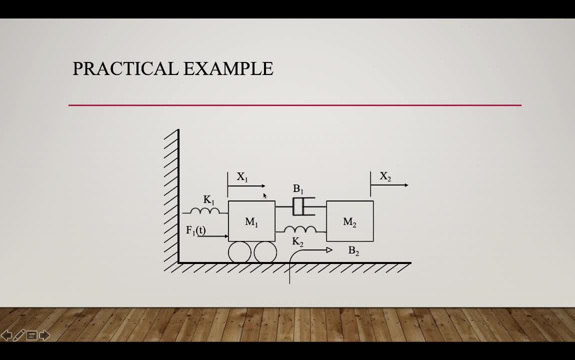 And there is some movement in it. There will be X1 movement in M1.. There will be X2 movement in M2.. So what do we have to do now? We have to develop a mathematical model. We have to develop a mathematical model of this system. 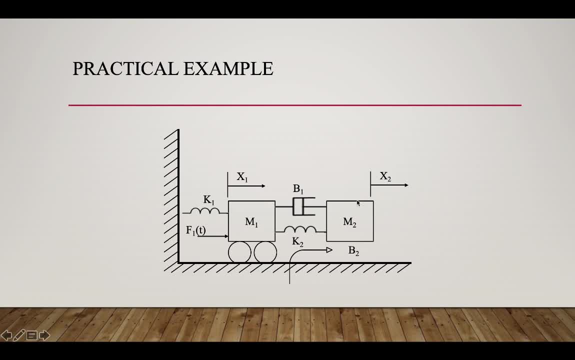 In which the input is F1 and the output is X2.. So, first of all, we will make its free body diagram. What is the free body diagram? All the mass elements. We will calculate the force applied on them, in which direction? 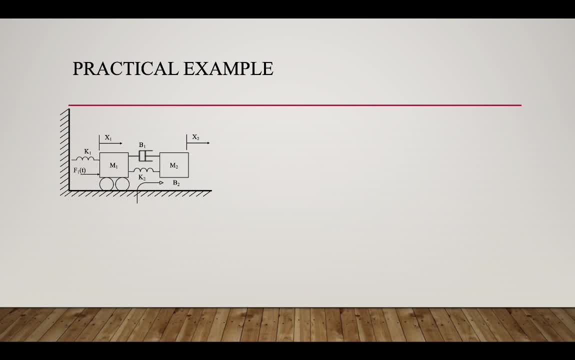 Then later we will balance them according to equilibrium. Okay, The sum of all forces on equilibrium should be zero. So first of all we will make the free body diagram of M1.. See what will be the movement in it. There will be X1 movement. 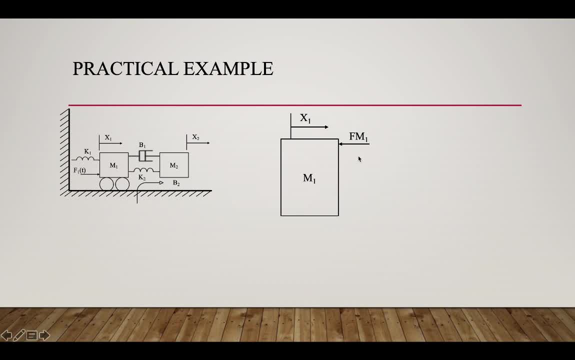 This direction will be on the right side. So how will the forces act on it? They will act on the left side. So FM1 is the force applied on it. due to its inertia, It is in the opposite direction. This is due to spring 1.. 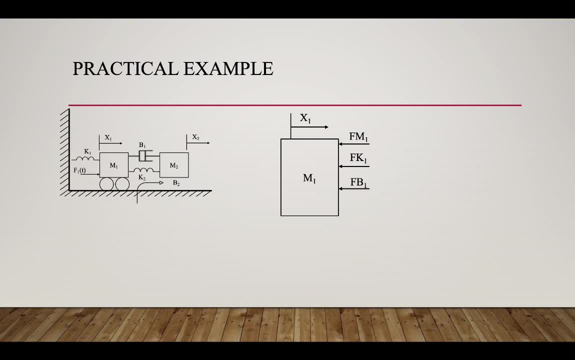 The force due to spring 1.. This is the force due to dashboard. This is the force due to spring 2, K2.. Okay, And the force which will make it move is F1.. It is applied on the right side. 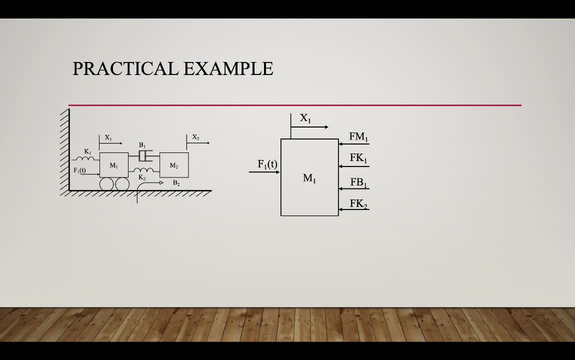 Rest of the forces are applied on the left side. So this is the free body diagram of this M1.. Okay, So we know what is the formula for force for mass, spring and dashboard. So we will write all the formulas. 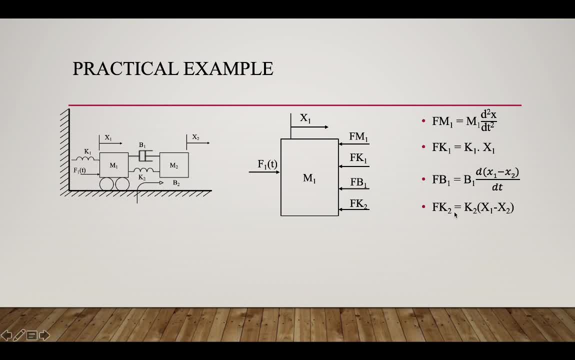 FM1, FK1, FV1, FK2.. Okay, Now we will put all these on equilibrium Means. sum of all these forces should be equal to this force. So we will write it in the form of equation.